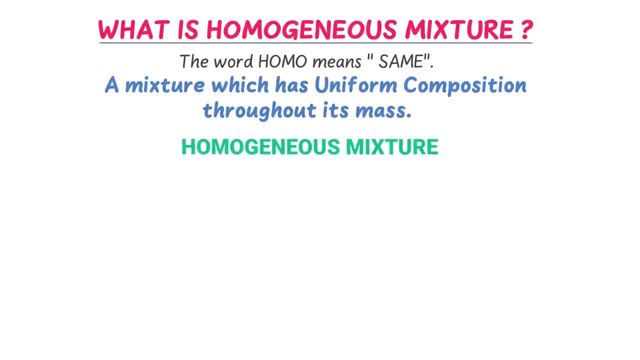 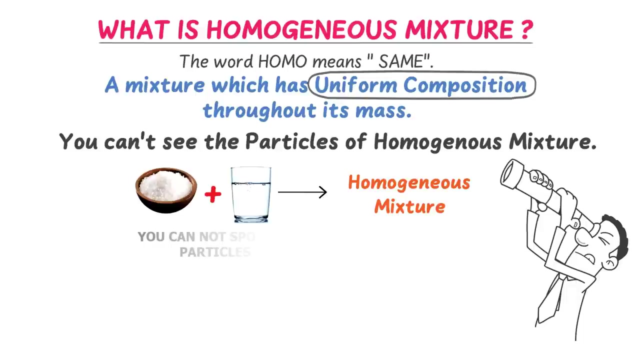 its mass is called homogeneous mixture. by uniform composition we mean that you cannot see or observe the particles of a homogeneous mixture with naked eye. the example of homogeneous mixture is: when you mix table salt plus water, you get a homogeneous mixture. remember that you cannot spot or see the particles of salt and water, and we therefore call it. 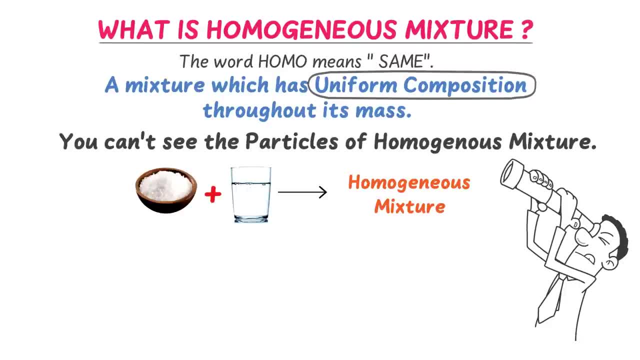 a homogeneous mixture. the second example of homogeneous mixture is air. we know that air is made up of different gases like oxygen, nitrogen and carbon dioxide. air is a homogeneous mixture because all these gases are combined together physically in such a way that they form a uniform composition throughout and we cannot see the particles of these gases. 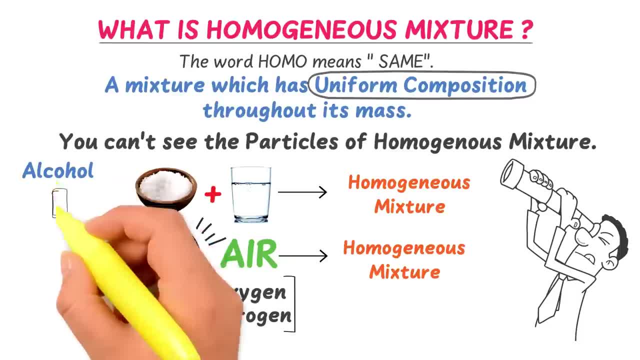 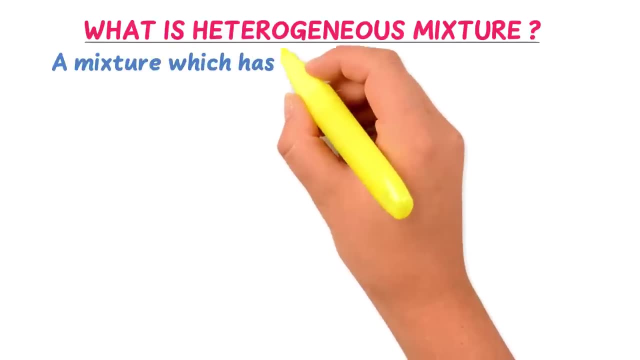 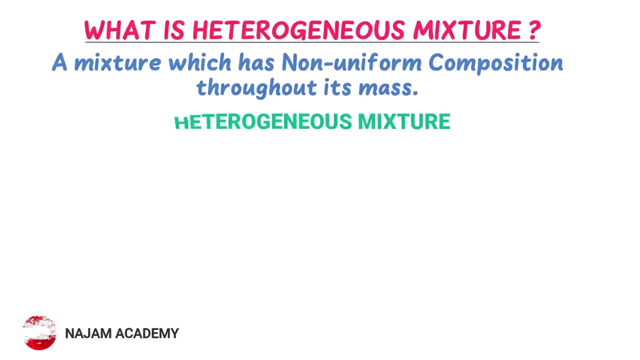 one last example of homogeneous mixture is air. we know that air is made up of different gases. last example of homogeneous mixture is alcohol. it has also uniform composition throughout its mass, and we therefore call it a homogeneous mixture. now, what is heterogeneous mixture? a mixture which has non-uniform composition throughout its mass is known as a heterogeneous mixture. 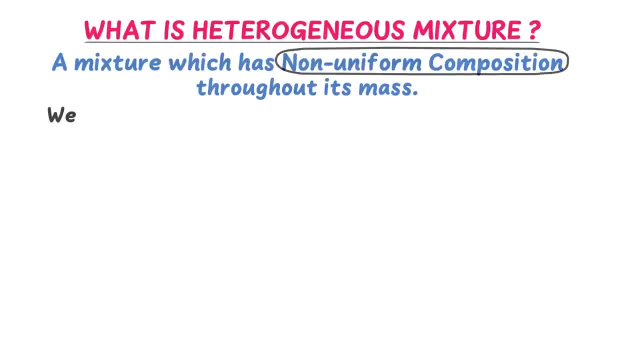 by non-uniform composition we mean that we see the particles of substances within the heterogeneous mixture with naked eye. the best example of heterogeneous mixture is salad. when you mix different vegetables physically, you get salad. secondly, you can easily recognize the ingredients of salad. the second example of heterogeneous mixture is 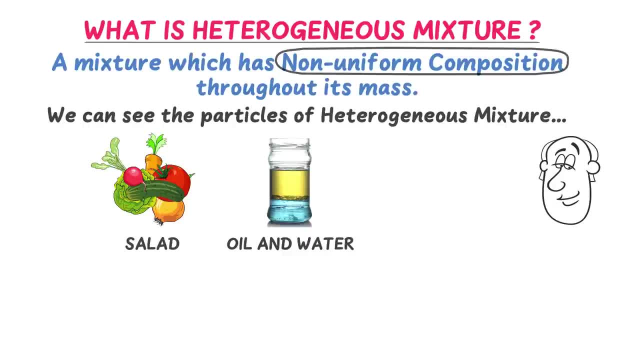 oil plus water. when you put some oil into the water, it is known as a heterogeneous mixture. you can recognize the layer of oil above the water. the third example of heterogeneous mixture is when you put small pebbles are sent into the water. it is called as heterogeneous mixture. you can.